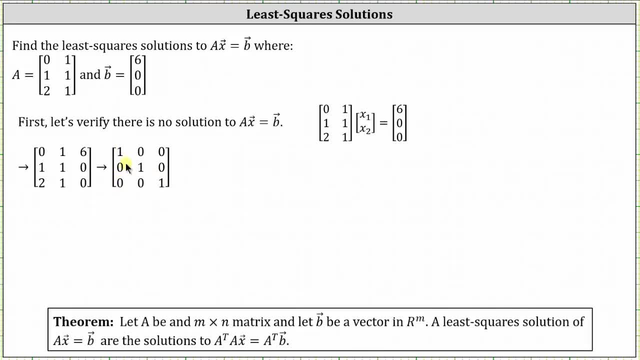 I've already written this in reduced row echelon form, Remember? the first column would be the coefficients of X one. The second column would be the coefficients of x two. The third column would be the constants. Notice we have a contradiction in row three. 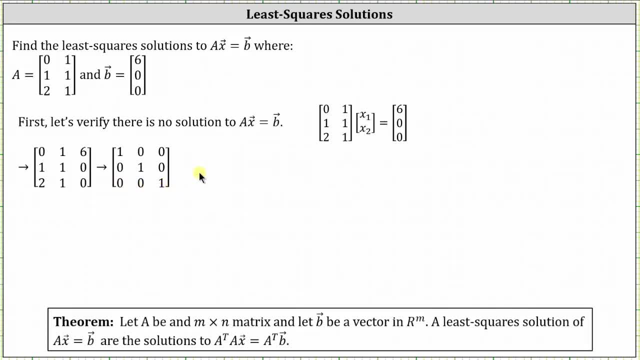 The third row indicates that zero equals one, which of course is not true, which verifies the equation a times vector x equals vector b has no solution. So now to find the least square solution, we need to find a transpose times a as well as a transpose times vector b. 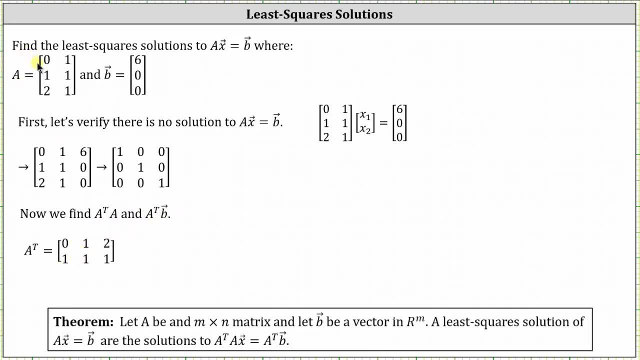 Remember to find a transpose. we take the first column of matrix a and this becomes the first row of a transpose, and the second column of matrix a becomes the second row of a transpose. So now we need to find a transpose times a. 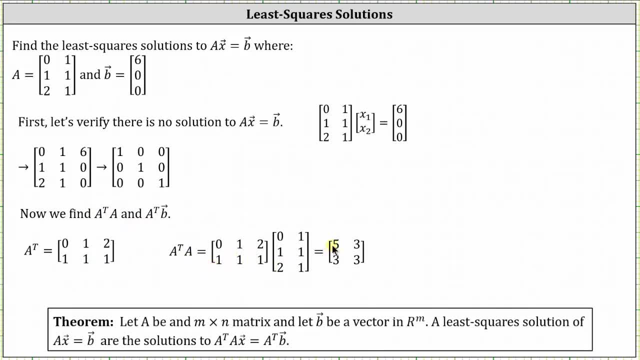 which I've already done here. The result is the two by two matrix, where the first row is five- three. the second row is three- three. You may want to pause and verify this product. Next we find a transpose times, vector b. 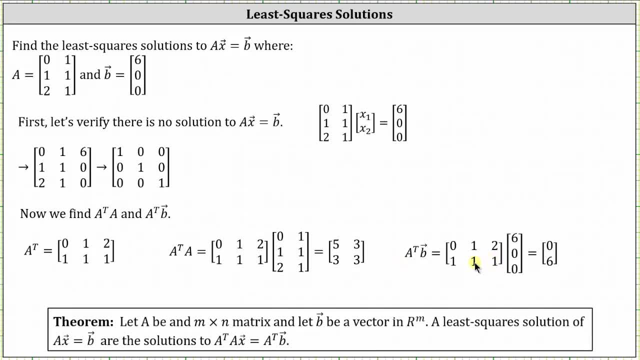 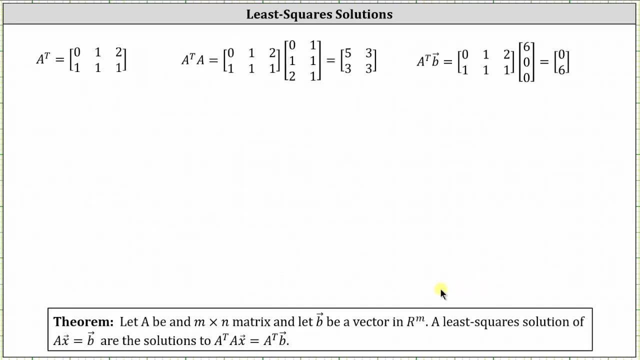 which, again, I've already done here. The result is the vector written as a column matrix with entries zero six. So now that we have a transpose times a as well as a transpose times vector b, step two is to set up and solve the equation. 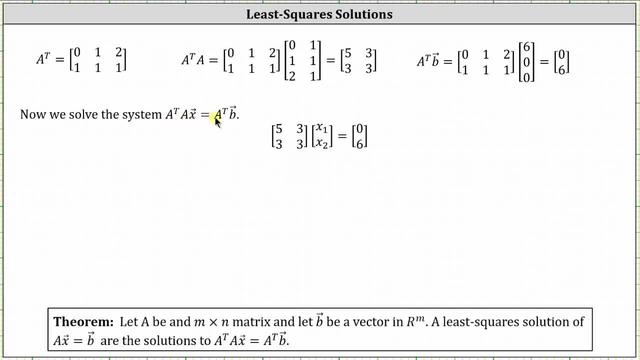 a transpose times. a times vector x equals a transpose times vector b, which gives us the following matrix equation. Next we write the corresponding augmented matrix and write the augmented matrix in reduced row echelon form. So for the augmented matrix, the first row is five, three zero. 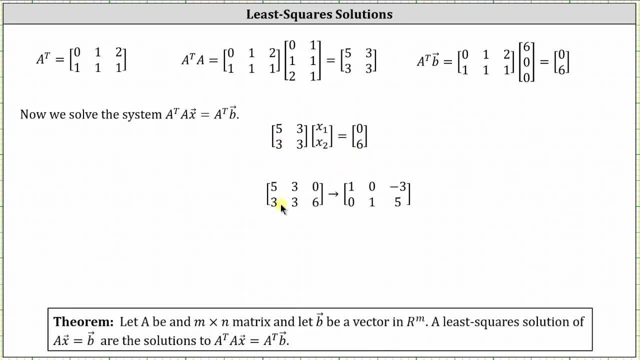 The second row is three, three, six, With the augmented matrix in reduced row. echelon form notice: x one equals negative, three x two equals five and therefore the least-squared solution is the vector negative- three, five, Instead of using vector x for the least-squared solution. 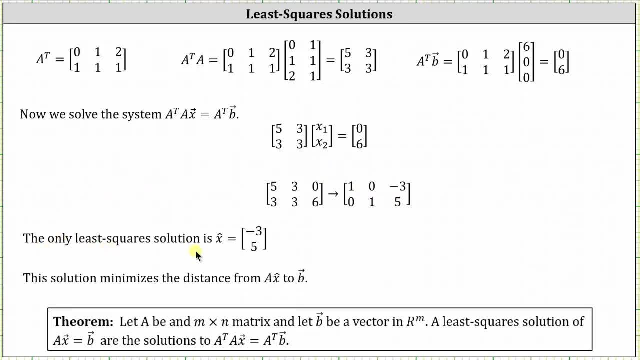 we often use different notation. In this case I'm going to use the vector x hat. So the least-square solution is x hat equals the vector x negative three five. Remember this solution minimizes the distance from matrix A times the vector X hat to vector B. 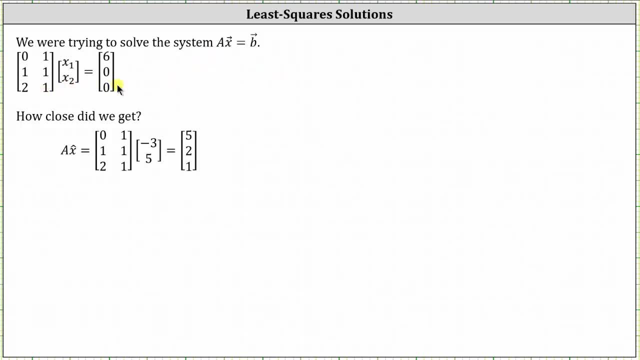 Going back to the original problem for a moment, if there was a solution to the equation matrix A times vector X equals vector B, there would have been a vector X one X two where matrix A times the vector X, one X two is equal to the vector six. zero, zero. 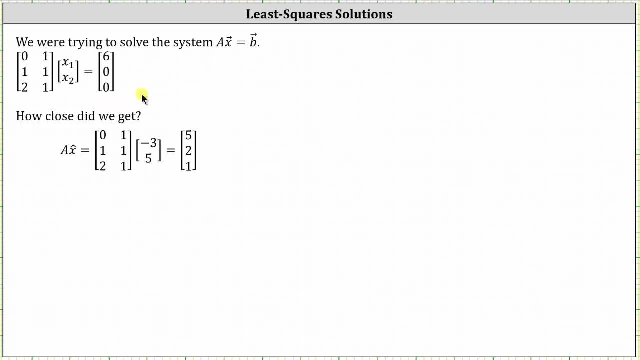 Because there was no solution, we found the least square solution which gave us the approximate solution of vector X. hat equals the vector negative three, five. Notice matrix A times the vector X hat is equal to the vector five, two, one, not the vector six, zero, zero. 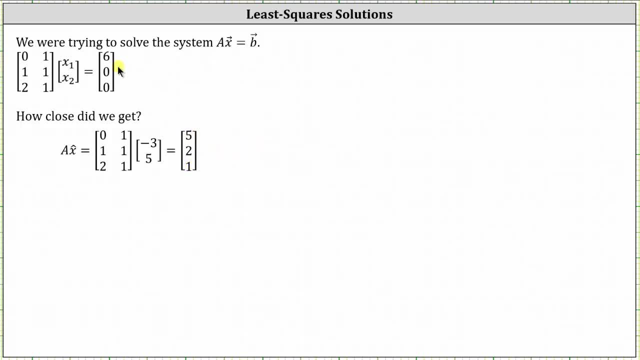 So the next question might be: how close is the vector five two one to the vector six, zero, zero? We can determine this by determining the magnitude of the difference of vector B and the vector resulting from matrix A times vector X hat, which is the vector five two one. 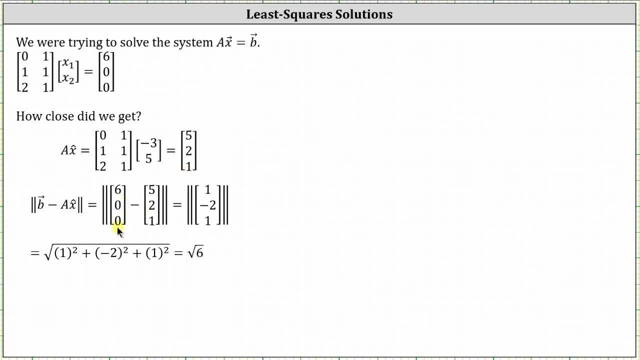 Which gives us the magnitude of the difference of the vector six zero zero and the vector five two, one which results in the square root of six. This indicates that the vector five two one is square root of six units from the vector six zero zero. Let's take a look at this graphically. 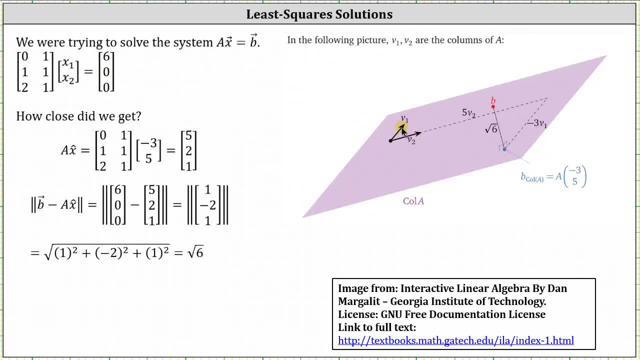 First, the purple plane is the column space of matrix A, where vector V one is the vector from the first column, the vector zero one two, and vector V two is the vector from the second column, the vector one one one. This is the terminal point of vector B. 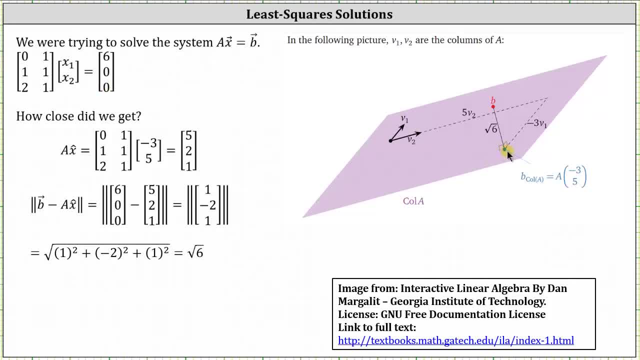 the vector six, zero, zero, and the blue point is the terminal point of the vector resulting from matrix A times the vector X hat, which is the vector five, two, one. We can also say the vector five two, one, or the vector resulting from matrix A times vector X hat. 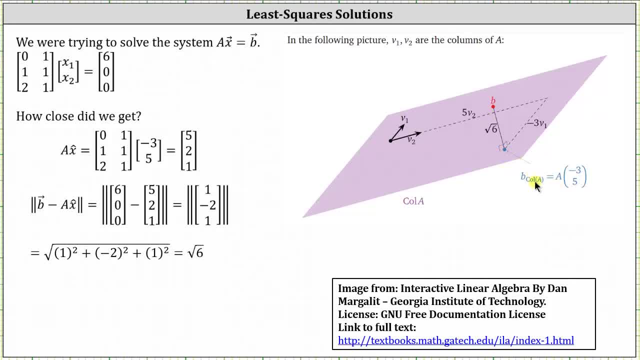 is equal to the vector B projected onto the column space of matrix A. And again, the distance from the vector five, two, one and the vector B is equal to this distance, here, the square root of six. So again, the least square solution minimizes the distance from matrix A. 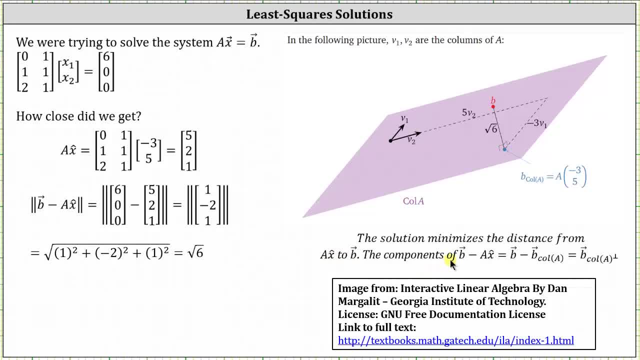 times vector X hat to vector B And the components of vector B minus matrix A times vector X hat is equal to vector B minus the projection of vector B onto the column space of matrix A, which is also equal to the projection of vector B onto the orthogonal complement.